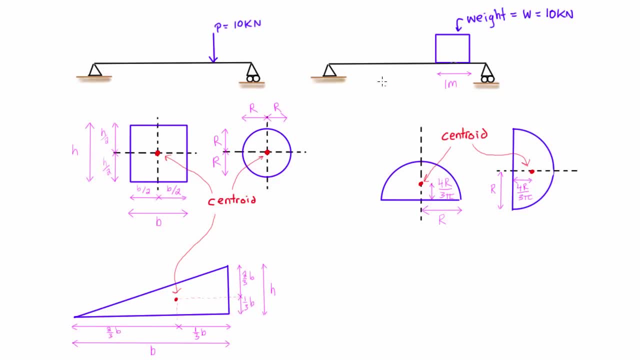 end of the object than the other. So if we go back up to our beam here with a square on it- assuming the square is of uniform thickness and material- then the centroid of that square is going to be right in the middle and that will also be the center of mass. Now we can use the 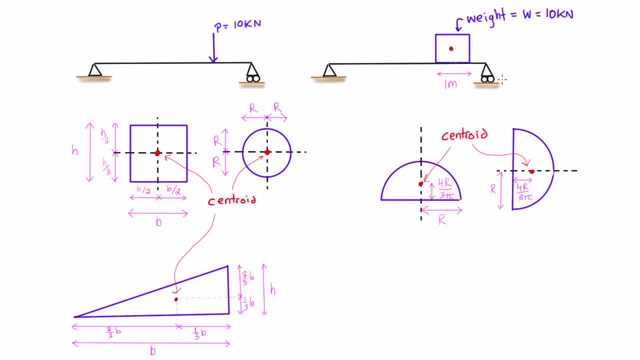 center of mass to solve for the reactions in a case like this. So let's actually change the dimensions here a little bit to make the numbers easier to work with. So we know that we have this. the weight of this whole object is 10 kilonewtons and its mass center is right here. 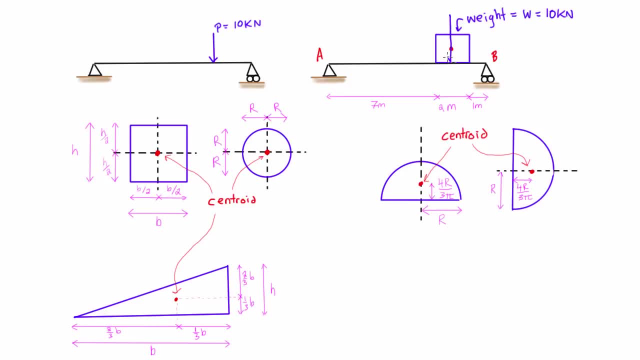 So basically we have a resultant force that's going to pass straight down right through that mass center or centroid of 10 kilonewtons And then we can just use that. we can actually see that the distance here from A to that line of action of that force is going to be 7 plus half. 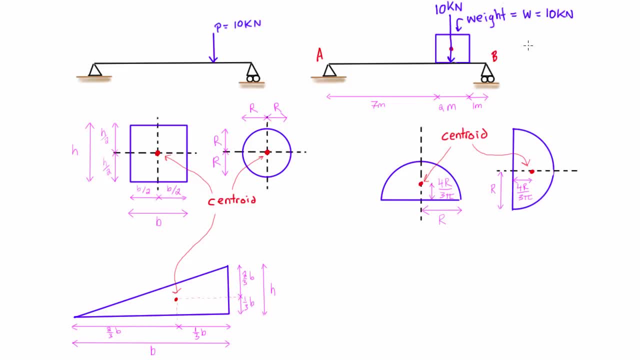 of this, so it'll be 8 meters. So if we take our sum of moments about A, then we're going to get what we have here. we have 10 kilonewtons times 8 meters is going to be equal to CY, or I guess BY sorry. 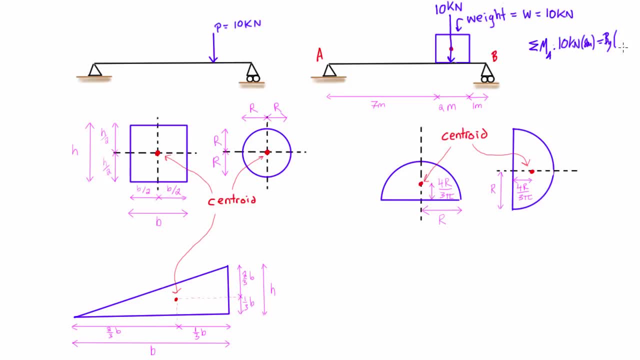 BY times this total distance, which is 10 meters. So if we just solve for that, then we'll just get that BY. here is equal to, it's going to come out to 8 kilonewtons, And then with the sum of forces in the Y direction, 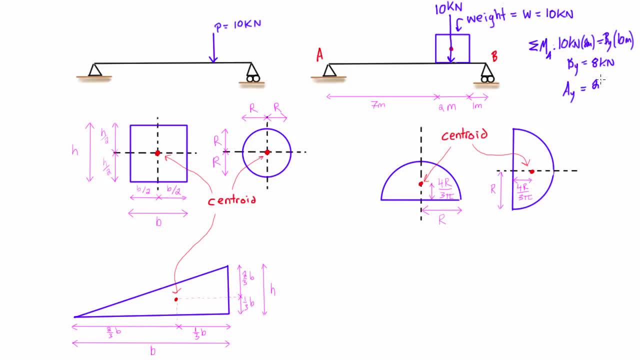 we're going to find that AY is going to be just that other, instead of gotten that other 2 kilonewtons. So there we go, by knowing where the centroid was of some shape, of a known weight. we were able to actually find the reaction forces at point A and B here. 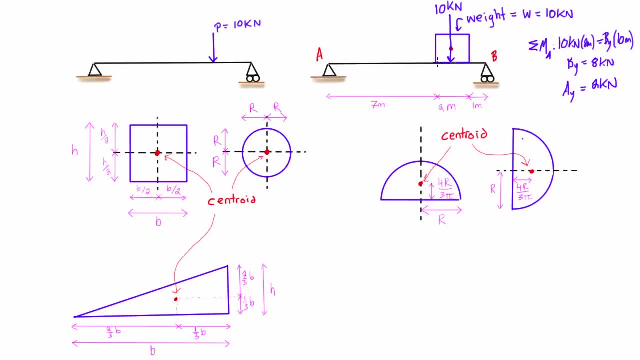 So that's pretty useful. If this shape would have been a triangle- that you know started in the same place and ended in the same place, but was a triangle shape- then it's centroid actually wouldn't be in the center, it would be shifted over to the right. 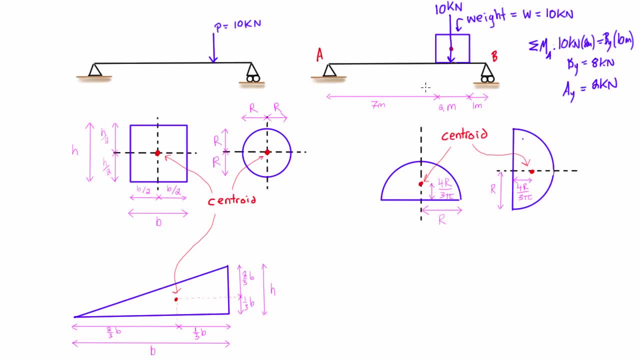 And if you look at this diagram it's actually one third of the way away from the tall side. So it would have been over to the right a little bit. and if that triangle also wouldn't weighed 10 kilonewtons, then the line of action of this force would have moved and that would mean